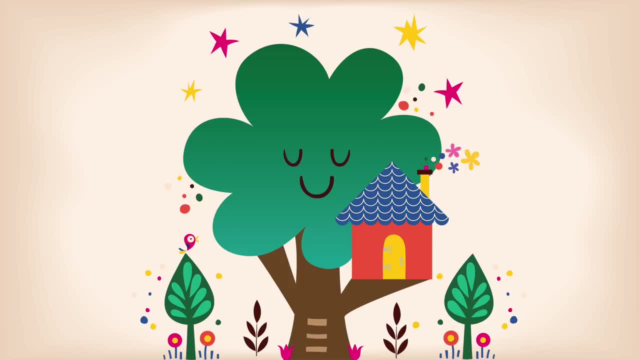 soft head. That's it. Super soft and gooey. Well done, Subtitles by the Amaraorg community. Now you're as soft as a melted marshmallow. Keep your eyes open And take a few big, deep breaths In through your nose And out through your mouth. Can you do two more? 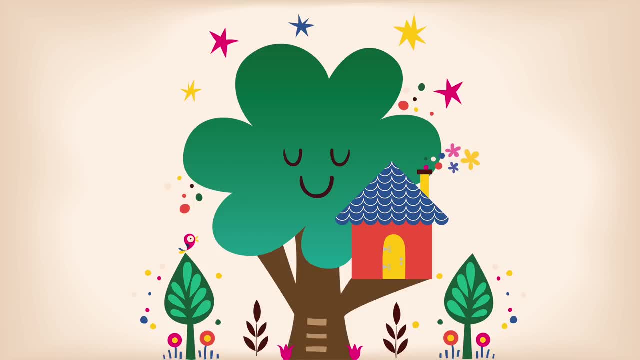 Wonderful, And on your next big breath out, Let your eyes close. Ahhh, That's it. Now you've made yourself as relaxed as can be. Your mind can play And take you on a really fun journey as you hear the words. 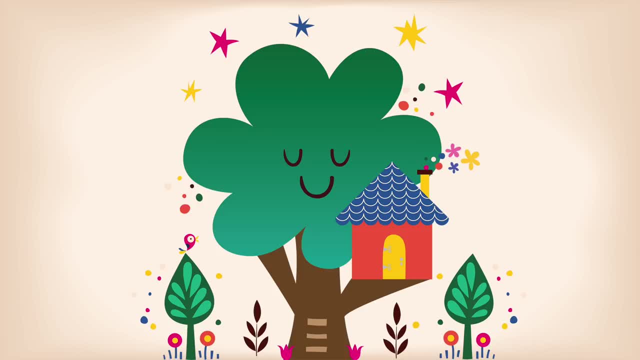 Ready Go. Subtitles by the Amaraorg community. Okay then Let's begin. You are standing in a beautiful garden. There are flowers everywhere. There are all sorts of colours: Yellow flowers, Blue petals, Green stems. Everywhere you look, You notice their 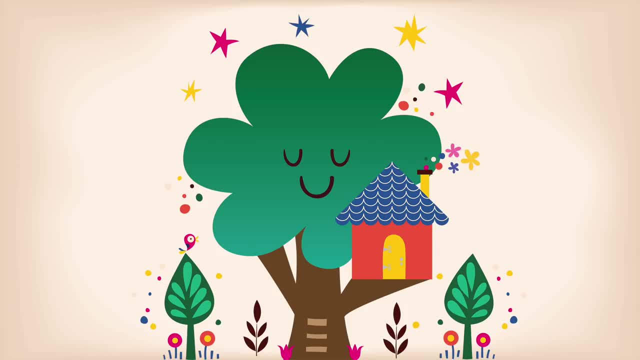 bright colors. Look, you notice their bright colours. They are all different sizes too. Some have tall, skinny stalks with big red heads. Others are small, tiny flowers, all bunched together in a clump. You breathe in and smell their sweet scent. 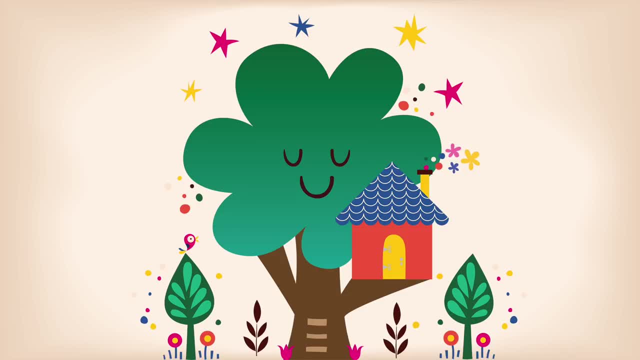 These flowers smell lovely. It's a warm summer's day. The air feels warm on your skin. You can hear a few birds whistling in the trees, singing and tweeting. Some sounds are far away. Others are closer to you. You start to walk through your garden along some round stepping stones that make a winding. 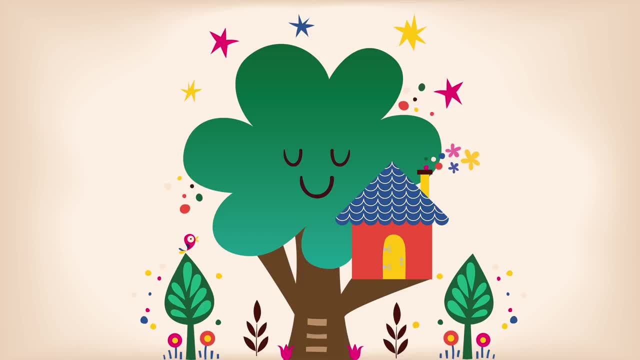 path down into the very back of the garden. The flowers line the sides of the path And you take in their colours And you smell the flowers along the way. Right at the end of the path is a big tree. The trunk is so wide you'd have to make your arms as wide as they go to reach the sides. 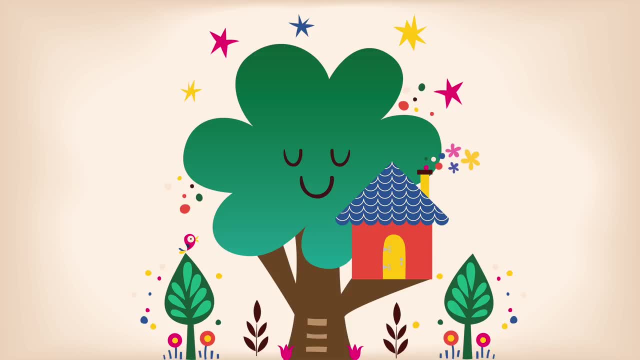 of it. You see there is a ladder made of rope and wooden steps dangling down the trunk. You see there is a ladder made of rope and wooden steps dangling down the trunk. You see there is a ladder made of rope and wooden steps dangling down the trunk. 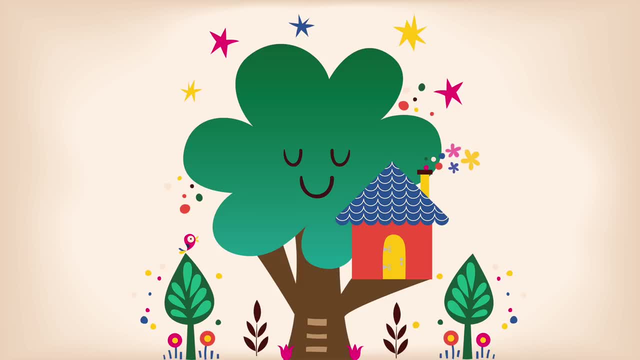 Hmm, This looks fun. you think Where will it lead? Which one will have the most amount of food? This is a house. It's a tree house, Like a real house, but in a tree. Who lives in there, you wonder? 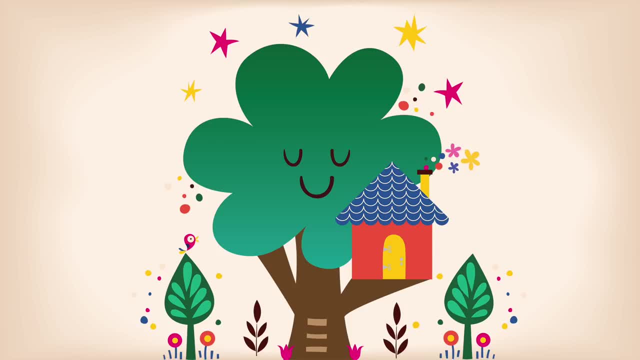 You turn the doorknob to open the door. Inside is a lovely big room with pictures on the walls, squishy cushions on the floor and a big armchair. What a cosy place this is. Sitting in the armchair is someone you know and love. 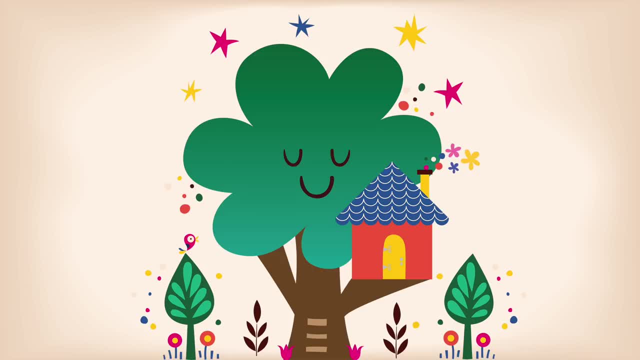 You decide who this is, as they are very special to you. They are smiling and very happy to see you. This person makes you feel very safe and happy. After giving them a big hug, you sit by them on the soft squishy cushions. 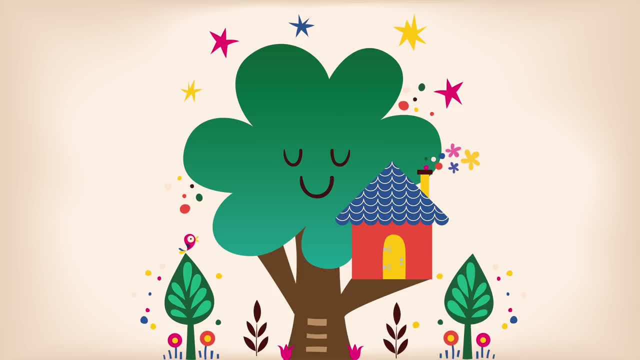 You take a moment enjoying being here and then you think of something, A question you have or something you've been wondering about. anything you like. This is a person you can ask anything, share anything. You know they love you and will understand and be happy to help you. 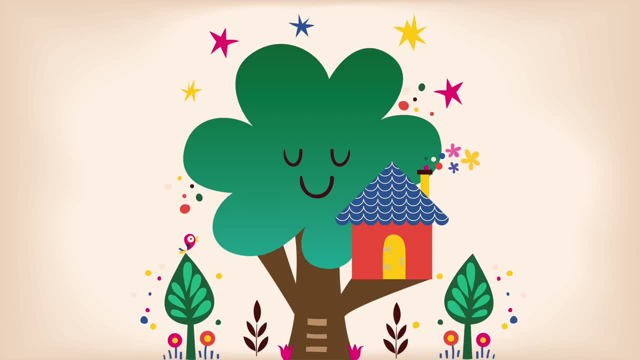 As you ask or tell them what it is you wish to say. they listen to you very carefully, Smiling kindly, Nodding gently And hearing your words. They understand exactly what you are trying to say. It feels so good to share your thought. 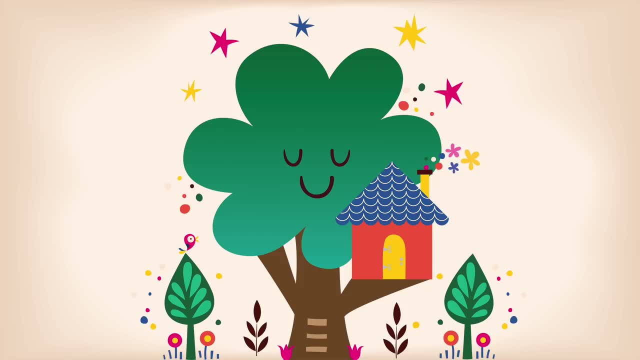 To share your thought and be understood, To have time to think and be listened to. When you have finished asking them your question or telling them your thought, maybe they say something back to you. Whatever they say makes you feel good about yourself. You understand better now. 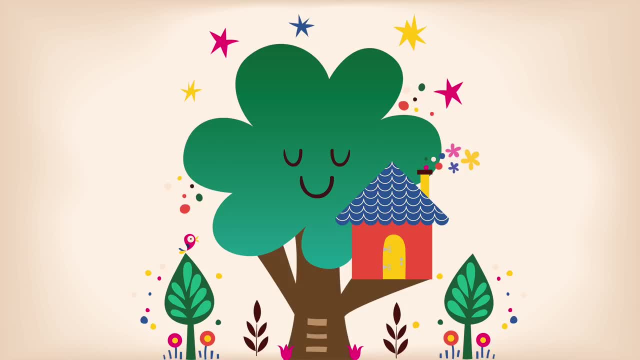 And feel glad for having shared, been listened to and understood. Talking to this person has been fun and helpful to you. They smile at you and you smile back. This is your magic treehouse And you can come back here and see your special person when you need them. 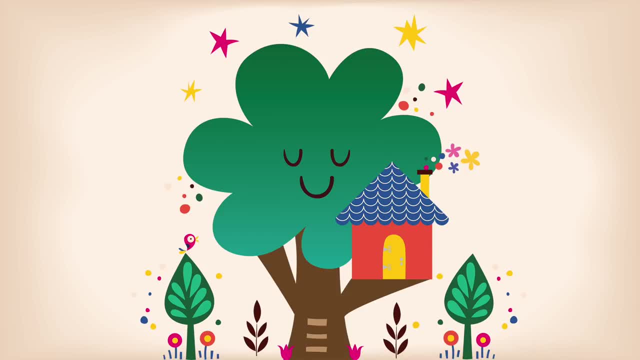 Now you know how much it helps to talk about things. You decide that next time something is on your mind, it will be a good thing to share it with someone you love and feel safe with, Feeling happy about having this special place. you say goodbye. 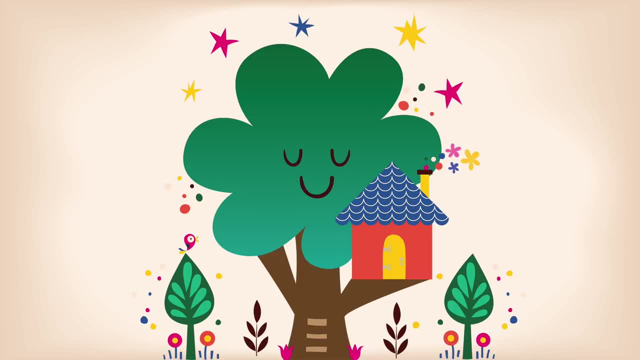 You walk out, Close your eyes, Close the door behind you, Return back down the big branch pathway And climb carefully down the ladder into the beautiful garden. As you stand there, the flowers all around in the warm sunshine, you take a moment to notice how you feel. 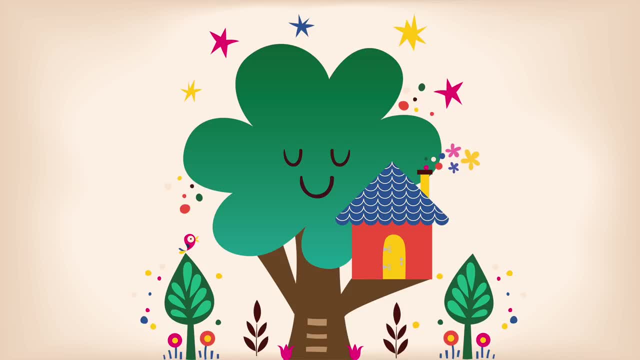 And you sigh, Feeling peaceful. Now we return. See if you can notice how your body feels sitting on a chair Or how the floor feels beneath you. Can you hear any other sounds around you? You take a big, deep breath And sigh out from your mouth. 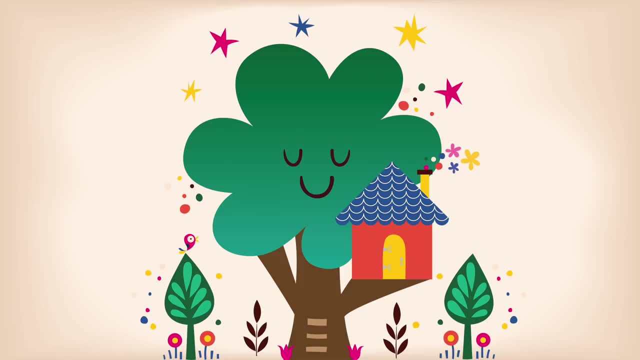 Have a stretch, if you like, And slowly open your eyes Now for just a moment. think about how you feel after that. Do you feel different to how you did before, Sleepy maybe? Or maybe you wanted to stay a bit longer in the magic treehouse. 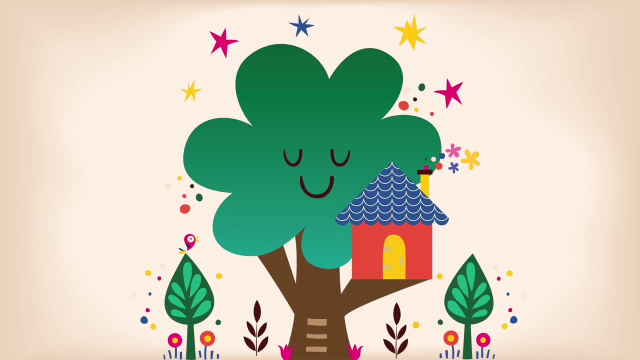 Maybe your mind was kind of busy when you were listening and you were thinking of some other things. That's okay. What's great is that you are learning how your mind works, And knowing your mind better will help you be the best you can be. 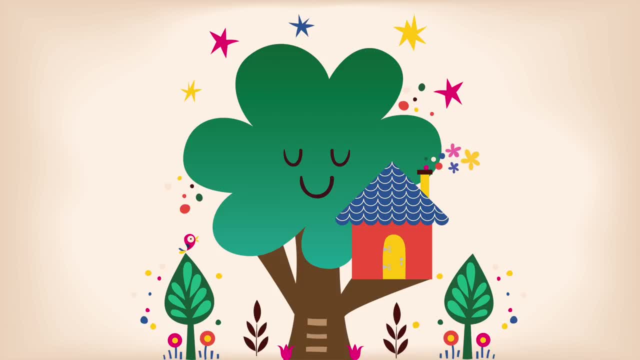 And, most importantly, have a very happy life. That's a good thing, don't you think? Well done you for listening And finding your very own superpower right there in your mind. This is Jamie saying peace out.